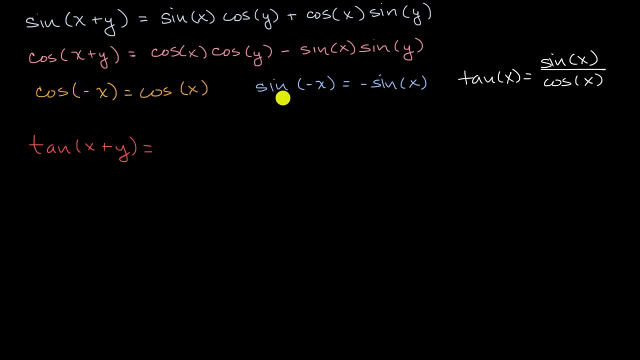 Cosine of negative x is equal to cosine of x, and that sine of negative x is equal to negative sine of x, And that, of course, the tangent of something is defined as sine over cosine of that something. Now, with that out of the way, 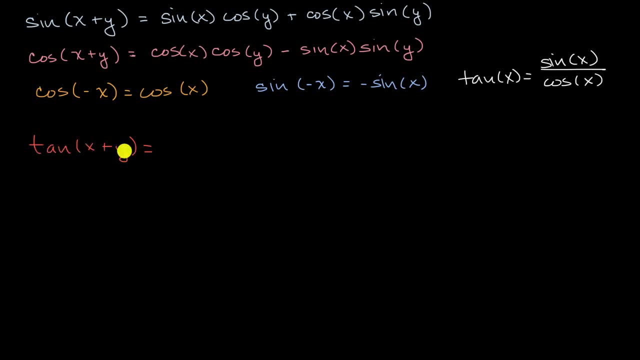 I want to come up with a formula for tangent of x plus y, expressed just in terms of tangent of x and tangent of y. You can view it as the analog for what we did up here for sine and cosine. Well, the immediate thing that you might recognize. 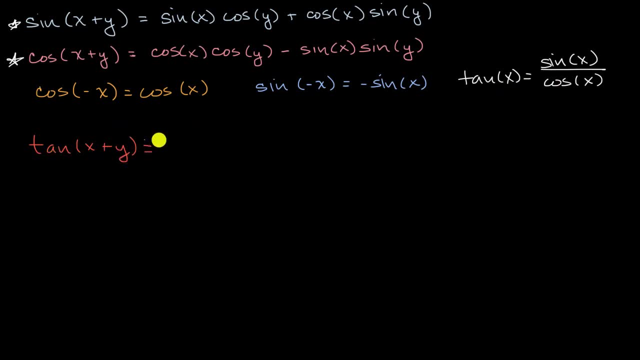 is that tangent of x plus y, based on the definition of tangent, is the same thing as sine of x plus y over cosine of x plus y. And what's that going to be equal to? Well, we know that sine of x plus y. 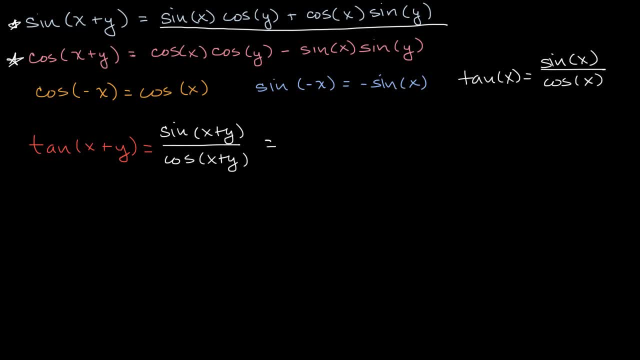 can be expressed this way. So let me write that down. So that's going to be sine of x, cosine y plus cosine of x, sine of y, And then, and actually, so that we can save a little bit of writing, I'm going to awkwardly write: make the line down here: 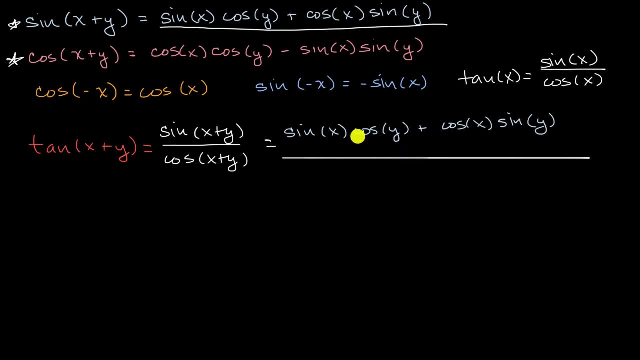 because we're going to put something here in a second, but I think you'll get the idea. So that's going to be that over cosine of x plus y, which is this expression when you just express it in terms of cosines of x and cosines of y. 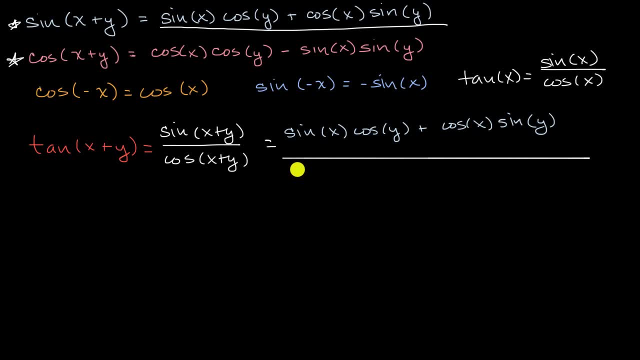 and sines of x and sines of y. So let me write it here. So you're going to have cosine of x, cosine y minus sine of x and then sine y. Now we want to express everything in terms of tangents of x's and y's. 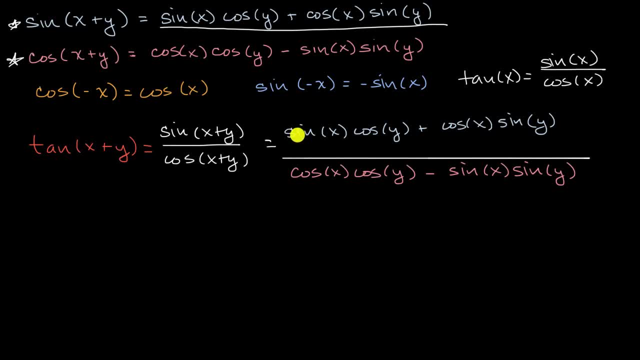 And so it might make sense here to say: all right, well, we know, tangent is sine over cosine. So what if we were to divide both the numerator and the denominator by some expression that can start to make the numerator and denominator express in terms of tangents. 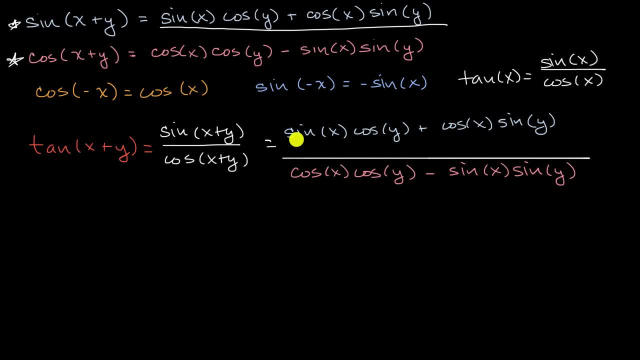 And I will cut a little bit to the chase here. So, in the numerator, what I can do is- and I'm gonna do this just in the numerator, and then I'm gonna do it in the denominator as well- I'm gonna divide the numerator by cosine of x. 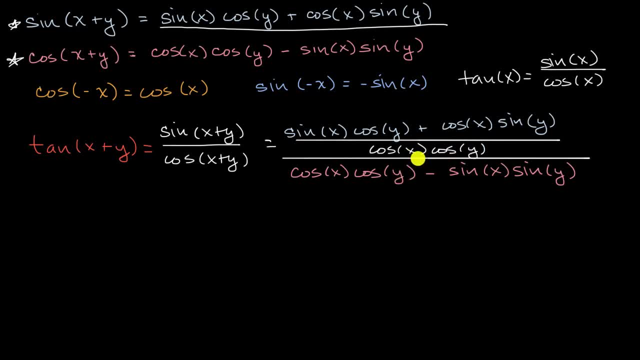 cosine y. And of course I can't just divide the numerator by cosine of x cosine y. That would change the value of this rational expression. I have to do that to the denominator as well. So I know this is a very complex looking fraction here. 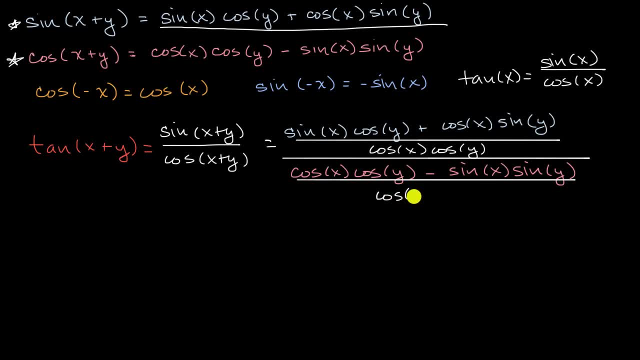 but it's going to simplify in a second. So I'm also gonna divide the denominator by cosine of x, cosine of y, And now let's see if we can simplify this in certain ways. On the in the numerator, we can see that this cosine y cancels with this cosine y. 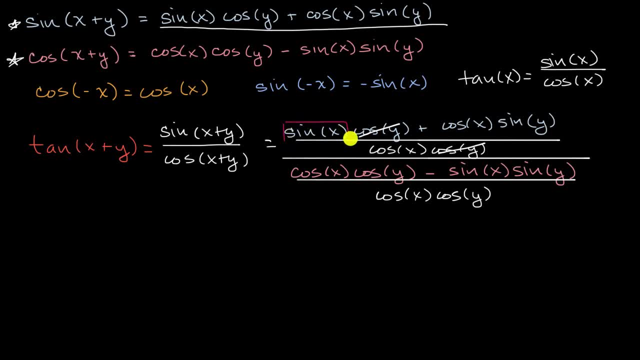 And so that first term becomes right in another color here. So this sine of x over cosine of x, And so the numerator, I can say this, is going to be equal to sine of x over cosine of x. So cosine of x is tangent of x. 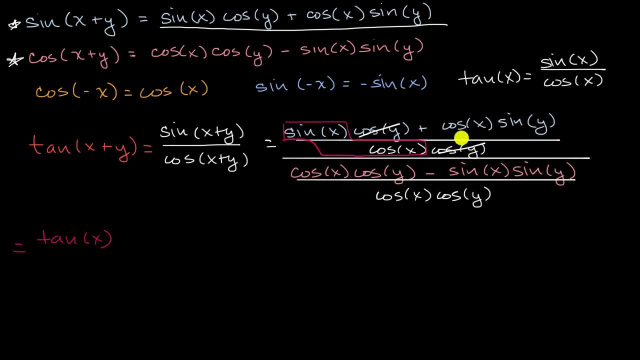 And then this second term. here we can see that this cosine of x cancels with this cosine of x, And so we're left with sine of y over cosine of y, which is of course tangent of y, So plus tangent of y. 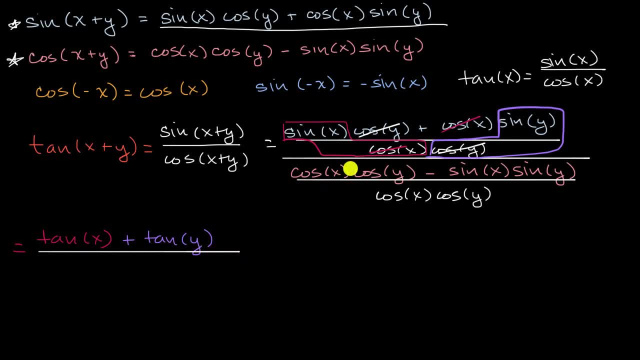 And then all of that is going to be over. Now we can look at the denominator, So this first term- here we can see the cosine of x cancels with the cosine of x and the cosine of y cancels out with the cosine of y. 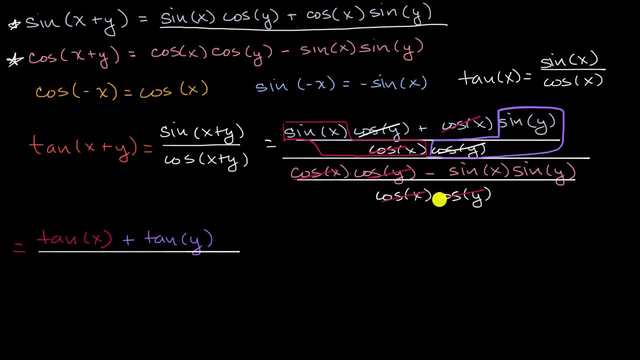 So you can view this first term here: when you divide by this cosine of x, cosine y, it just becomes one, And then we're going to have the minus. And now this second term is interesting: We have sine of x over cosine of x. 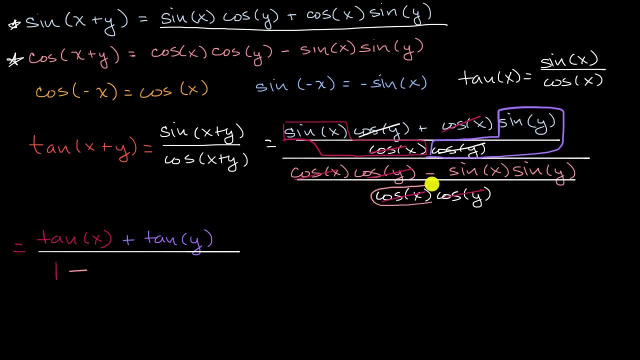 sine of y over cosine of y, So sine of x over cosine of x, That over there is tangent of x over cosine of y, tangent of x, and then sine of y over cosine of y, that's tangent of y. So this is going to be tangent of x times tangent of y. 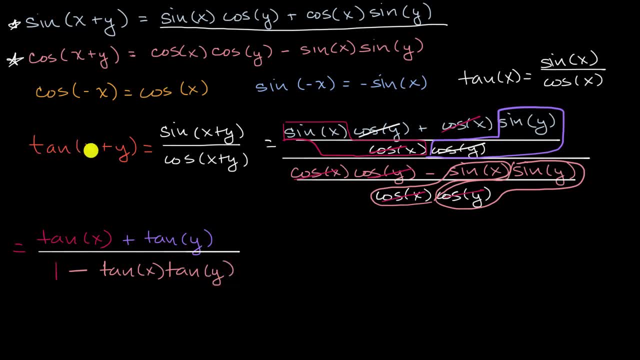 And just like that we have come up with an expression for tangent of x plus y that just deals with tangent of x's and tangent of y's. Now the next question. you might say: well, all right, that's great for tangent of x plus y.